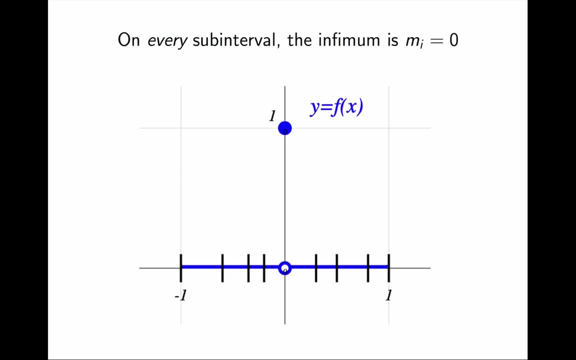 On any subinterval, no matter what, the infimum is always going to be 0.. It does not matter if the partition includes 0 or not. Therefore, all the lower rectangles have height 0, and the lower sum is 0 for EVERY partition. 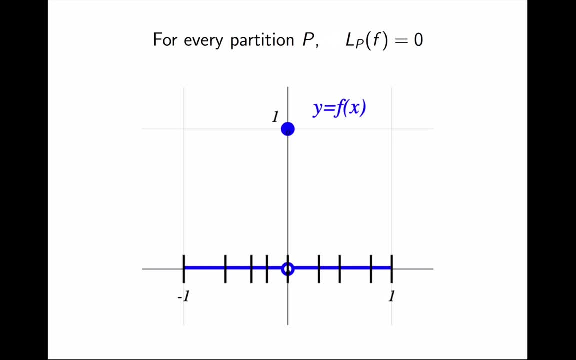 EVERY lower sum is 0.. We can calculate the lower integral with this information. The lower integral is the supremum of all the lower sums, the supremum of the set of all lower sums, But that is just the set with one single element: 0.. 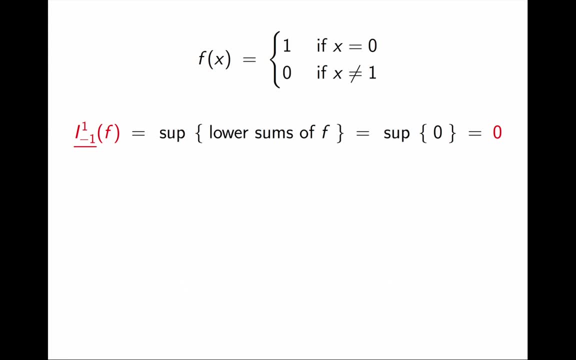 So the lower integral is 0.. Let's look at the upper sums. They are more interesting. I have an arbitrary partition here. As you know, the upper sum is the area of the rectangles above the graph in green in this picture. 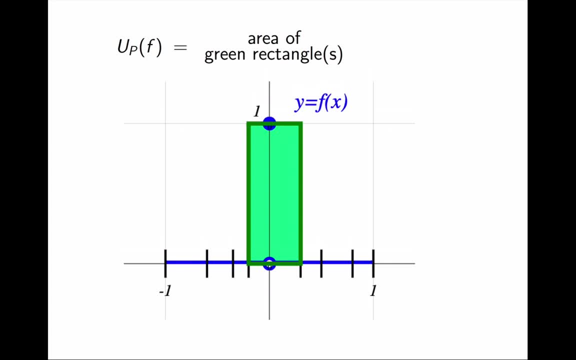 In this case there is one rectangle with height 1.. It is the rectangle for the subinterval that contains the value x equals 0. All the other rectangles have height 0, and are not contributing. Notice that 0 is not a point in this particular partition. 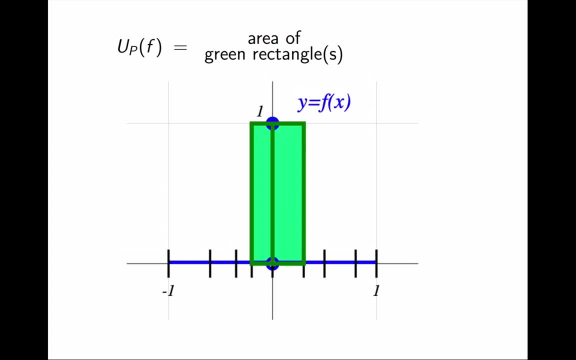 If I choose to add 0 to the partition, it will just split the one rectangle in two, but it won't change the upper sum. Notice also that the extra points in the partition are not doing anything. They do not contribute extra rectangles. 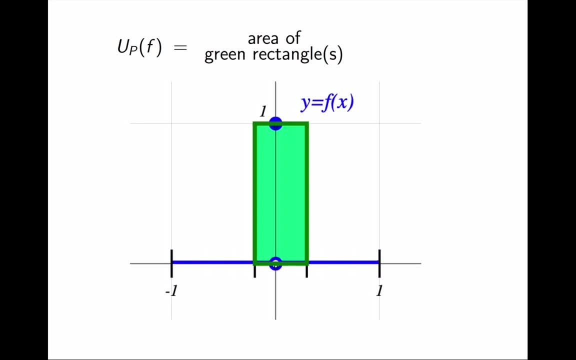 they do not change the upper sum, So I will ignore them. Okay then, The upper sum is the area of this one rectangle. the area is height, which is 1, times width. And what is the width? It can be bigger or smaller. 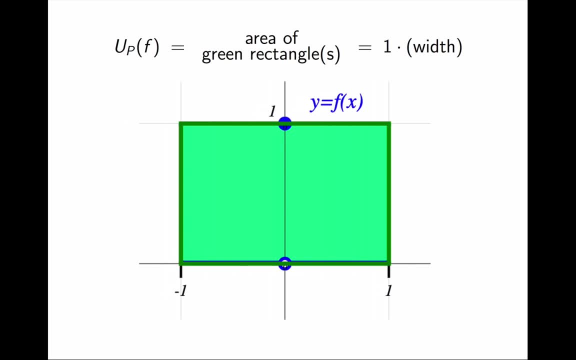 It can be as big as 2, if I use the simplest partition, just the points minus 1 and 1, and nothing else, And it can get as small as we want, but always remain in positive. It can also take any values in between. 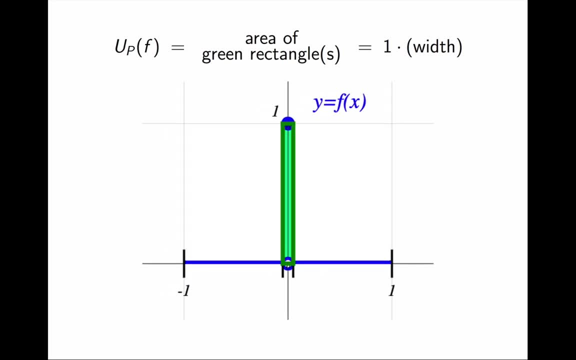 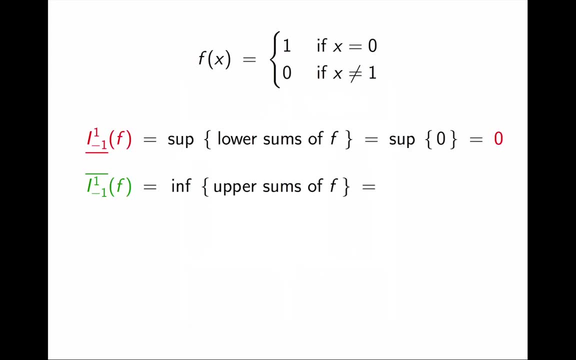 so anything between 2, inclusive and 0,, not inclusive. Great. we can now calculate the upper integral. It is the infimum of the set of upper sums. The set of upper sums is the interval from 0, not included.